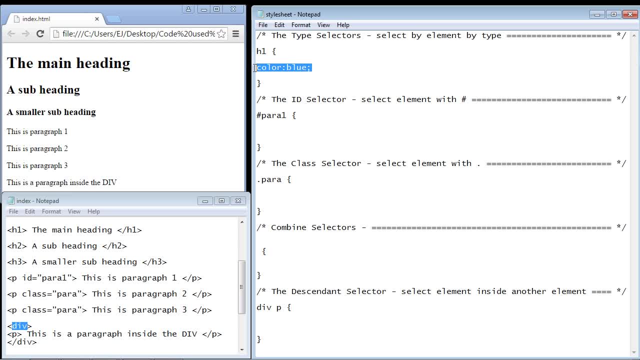 and we're just gonna change the color of the text. The point of these videos is not styling. we're actually talking about this part, the selector. So let's go ahead and save this and we'll refresh our page and there you can see, we've got our blue. 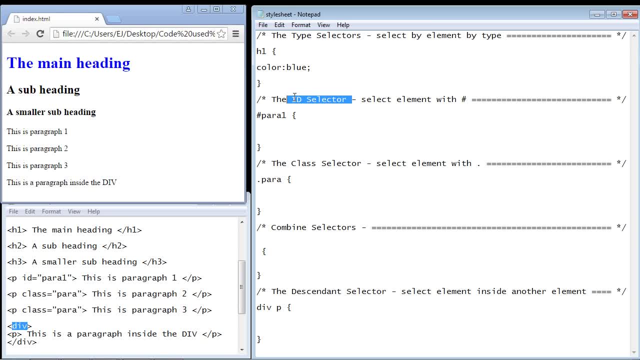 text. Now, the next major selector that we've been talking about, of course, is the ID selector, and that, of course, is where we select the element with the hashtag by ID and we put that right here and in this paragraph element we said: ID equals para1 and remember, with the ID, we usually will not be reusing this in. 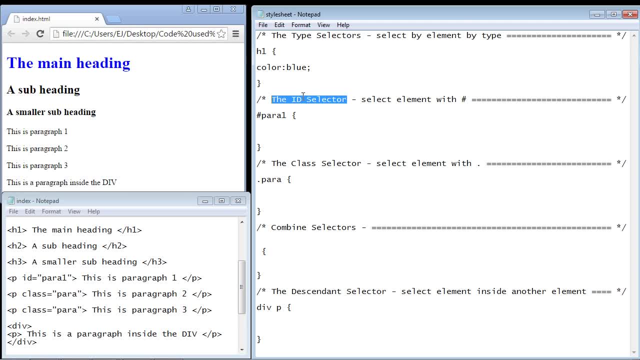 other elements. It's usually specific to one element that we want to style, So let's just go ahead and change the text to green and we'll refresh our page, and there you can see, we've got our green text. Now the next major selector of 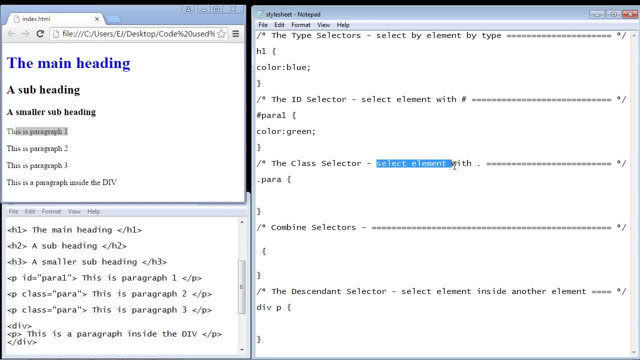 course, is the class selector, and you will remember that we always select that element with a dot. That is how we select it in CSS, and you can see that right here: dot para. and the nice thing about this, of course, is we can also select the element with a dot. That is how we select it in CSS, and you can see that right here: dot para. and the nice thing about this, of course, is we can. 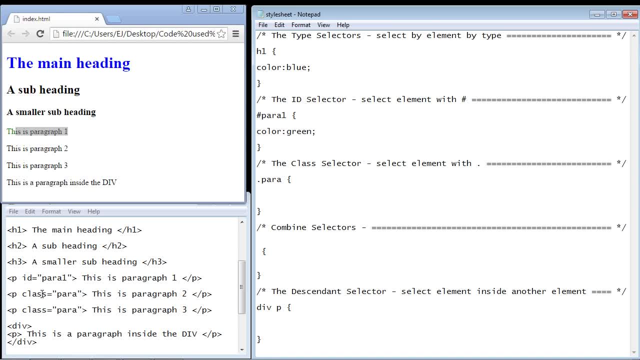 reuse the class over and over again in other elements, and that's what I've done here. This paragraph element is using the para class and this paragraph element is using the para class, So we can reuse this over many, many times, and all we need to do again is use that dot. So let's go ahead and change the color of. 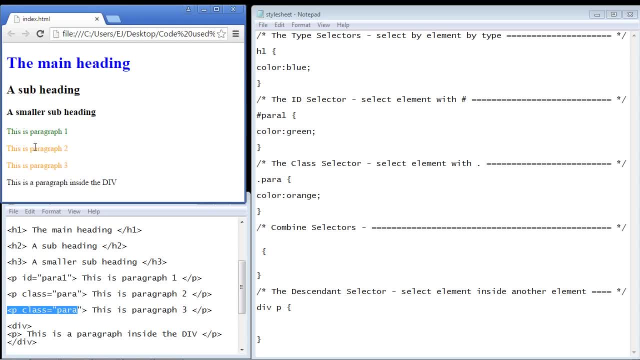 the text to orange. We'll refresh our page and there you can see we have our orange text now. Now we can also combine selectors, So we can put multiple selectors in one of our rule sets. So let's do that, Let's take, let's take the h2 and we'll put that in here. and of course, we need a. 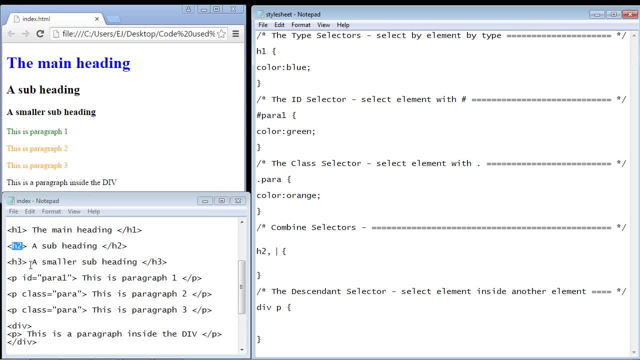 comma. That's how we separate when we use multiple selectors. and let's go ahead and we'll style against the h3 and we can reuse any other selector we want. We can reuse the ID selector. So let's put that in here as well, and then what we'll. 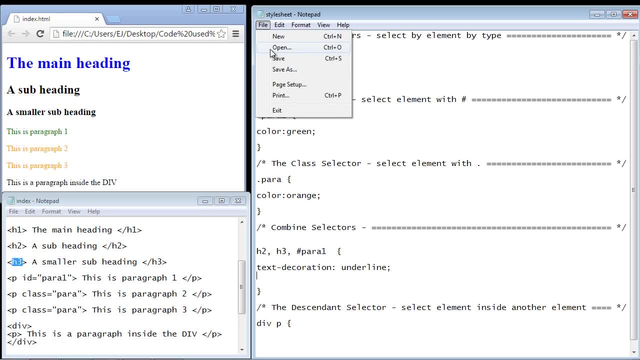 do is we'll underline the text. So we'll go ahead and refresh and there you can see the text in. the h2 and the h3. are now underlined, as well as the paragraph element with the ID. Now the key again is: you want to use that comma. If you don't, CSS will get confused and